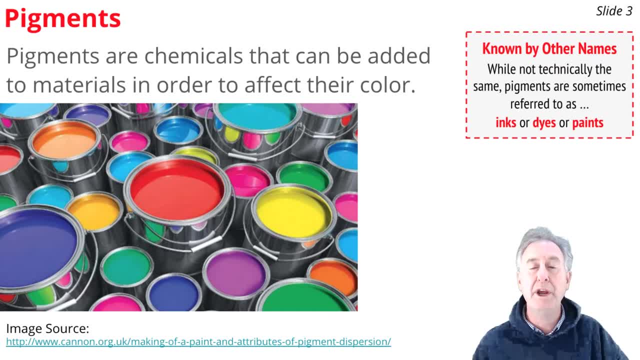 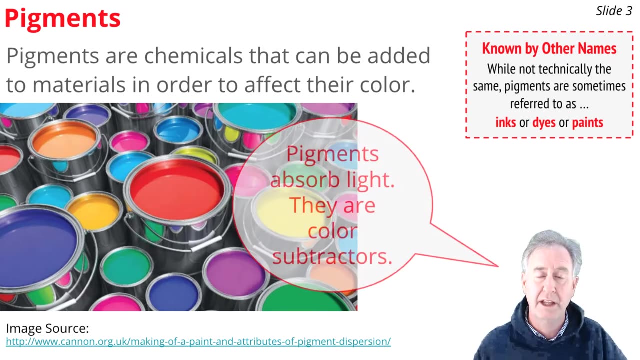 and a pigment are not exactly the same thing. they operate in much the same way. They're a chemical imparted to a material to affect its color appearance and they operate on the basis of they subtract specific colors of light from the light that lands on the object. They absorb light. 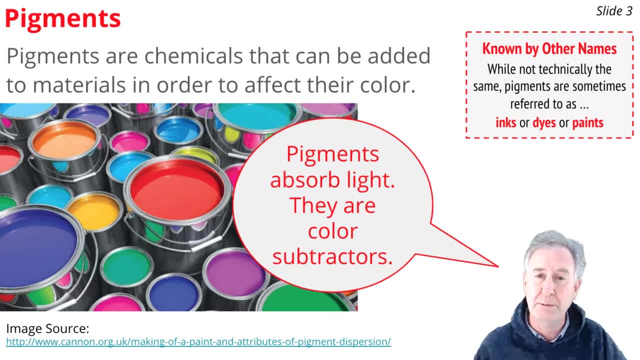 and because they absorb light, they operate under the principles of color subtraction. So we're going to be talking a lot today in this video about pigments and color subtraction. So we've been talking quite a bit about light in these videos. Now we're going to be talking 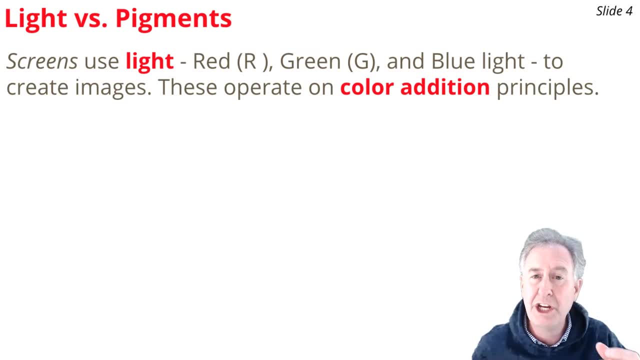 about pigments, And pigments and light are different. They might share some similar names, but they're different. So here's a way to explain it: Screens like this- computer screen, a phone screen, a television screen- they use light- Red, green and blue light- with varying intensities. 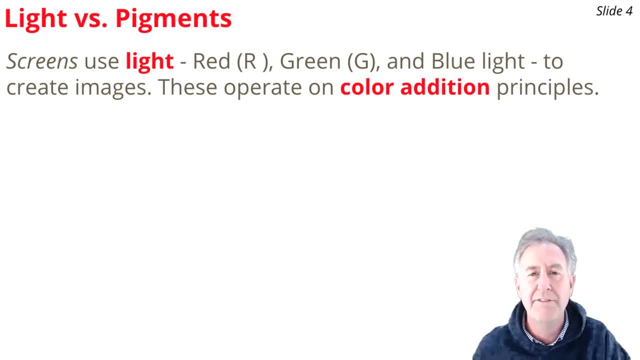 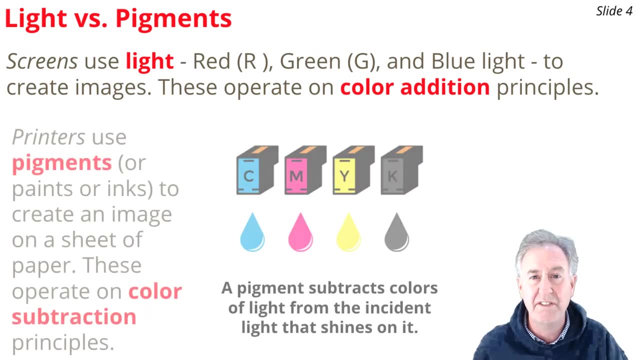 of color subtraction makes kä shuts or Columbians find their pigments are different. but again, with the color subtraction process, the color doesn't create an image, but instead it creates an image. The light adds together, follows rules of color addition. Now that's quite. 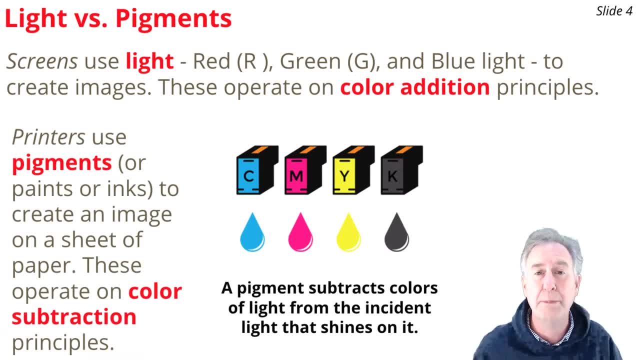 different than pigments, because pigments are chemicals. It's stuff that printers use. Printers use pigments and they impart the pigment to a white sheet of paper And when the light lands on the paper, the pigment that is there absorbs, subtracts or takes away one or more colors of. 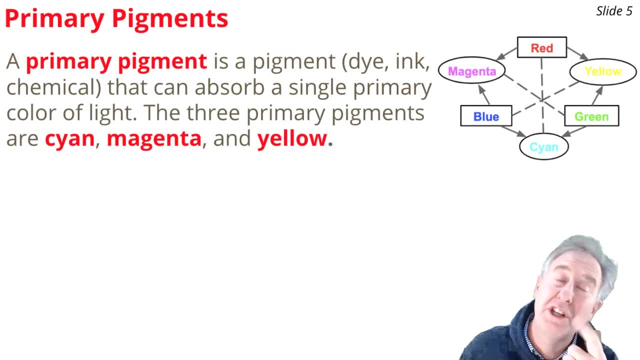 they're absorbing light. so we've been using this little schematic quite a bit in these videos. the schematic works for light, but it also works for pigments. when we use it for pigments, here's how we use it. there are three need to know them. primary pigments: they are cyan, magenta and yellow. you see them in the. 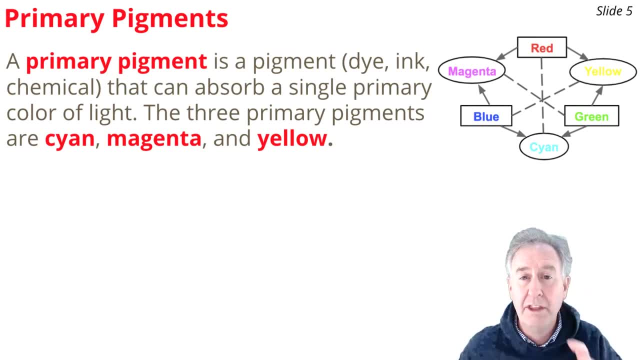 ovals on the schematic diagram above my head. now these primary pigments are called primary pigments because they absorb one single primary color of light. here's how you can find out how it works. cyan is our first primary pigment. you find it on the color wheel. it's right at the bottom in the oval. it absorbs the and exercise helps the pigment- 복 помог, Karola- would show different these different marks as well. So we're talking about light jets that are loosingуетal and it can cause wind insulting eggs, andalin. so none of these make, verily, can, candles. So one of each type of pigment is killed and no other can not live in the moment. So 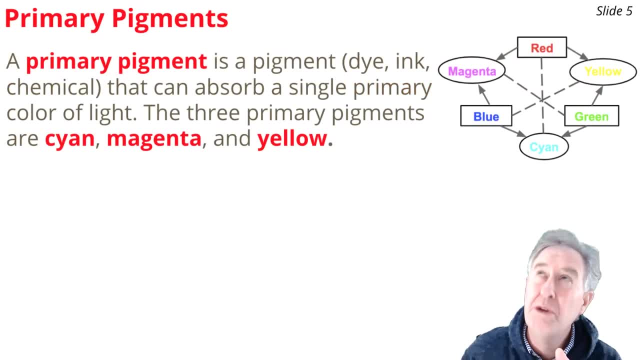 because they're absorbing light. So we've been using this little schematic quite a bit in these videos. The schematic works for light, but it also works for pigments. When we use it for pigments, here's how we use it. There are three. you need to know them. primary pigments: They are cyan. 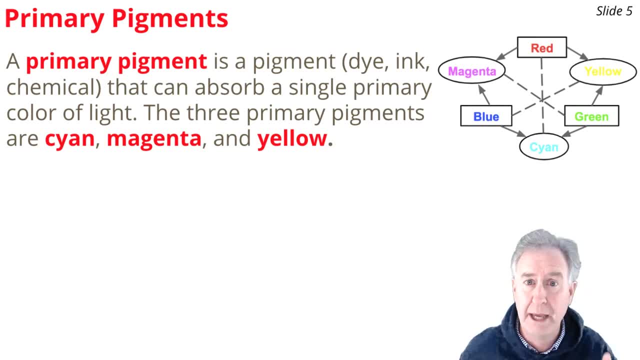 magenta and yellow. You see them in the ovals on the schematic diagram above my head. Now, these primary pigments are called primary pigments because they absorb one single primary color of light. Here's how you can find out how it works. Cyan is our first primary pigment. You. 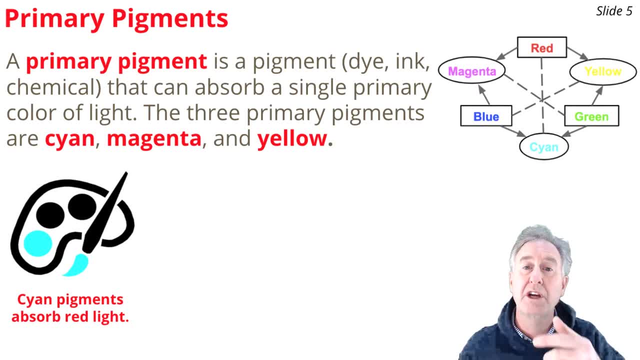 find it on the color wheel. It's right at the bottom in the oval. It absorbs the color of light that's across from it. Cyan pigments absorb red light. Our next pigment is magenta. You see it on the color wheel. Look right across from it. What does it absorb? Magenta pigments absorb red light. 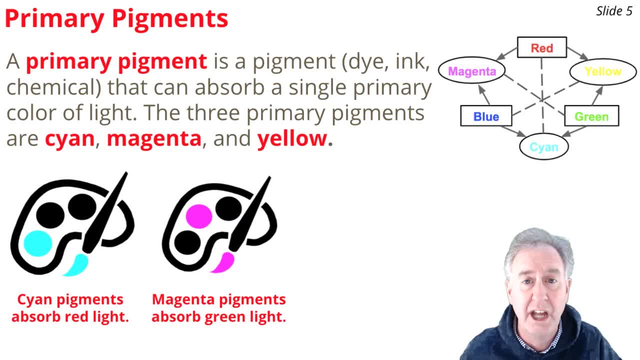 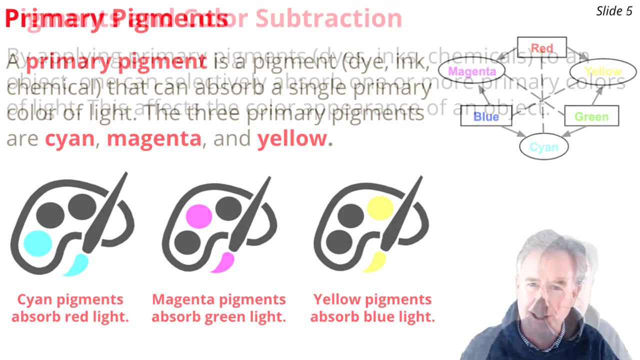 Magenta pigments absorb green light whenever green light shines on an object with magenta pigment. And finally, yellow pigments: They absorb whatever's across from them, That's blue light. So there's your three primary pigments. Each one absorbs a single primary color of light. 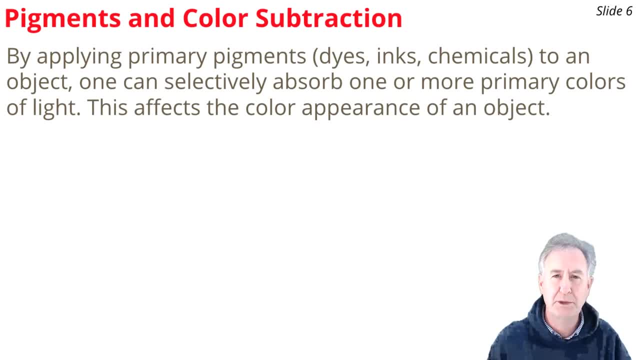 So here's how this idea- a color subtraction in pigments- works. When you apply a pigment to an object- a sheet of paper, a shirt, whatever it is- that pigment will absorb a single primary color of light. So let's just say we have a shirt and magenta pigments in the shirt And we shine. 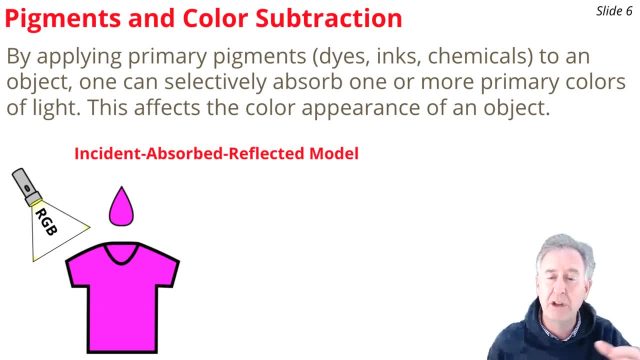 white light down on the shirt. White light's red and green and blue light combined And when it hits that shirt- you remember the color wheel- the magenta will absorb the green light. So if you start with red, green and blue and green gets taken away, there's two colors remaining: Red and 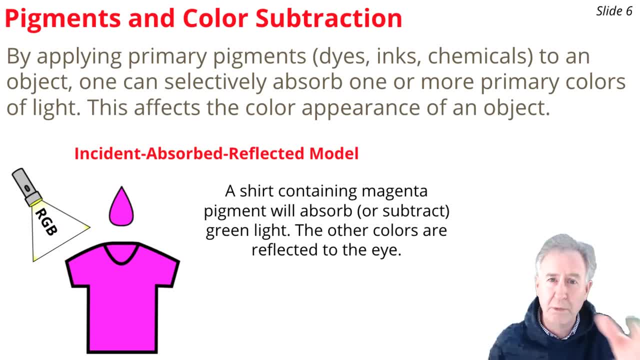 blue reflect off the shirt to your eye, and your eye and your brain work together to say: hey, that's a magenta shirt. In terms of a color subtraction equation, it would look something like this: You start with red plus green plus blue, But then the shirt takes away the green, so we subtract it, Then do the math. 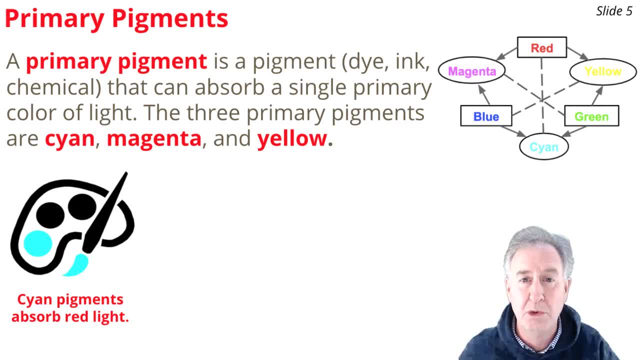 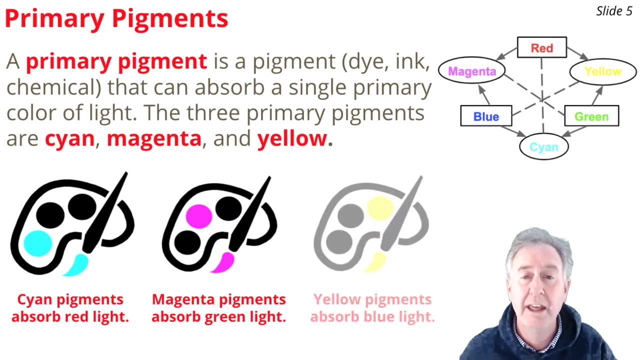 color of light. that's across from it. cyan pigments absorb red light. our next pigment is magenta. you see it on the color wheel. look right across from it. what does it absorb? magenta pigments absorb green light. whenever greens absorb green light, light shines on an object with magenta pigment. And finally, yellow pigments. They absorb whatever's. 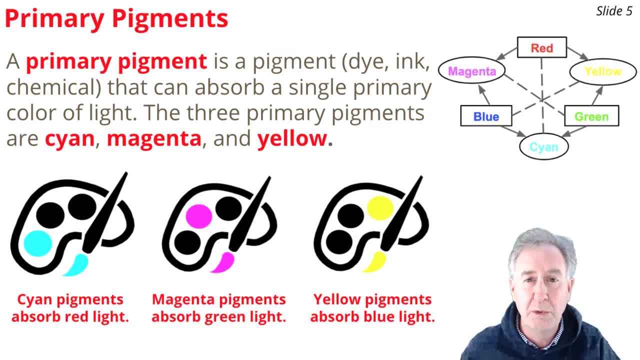 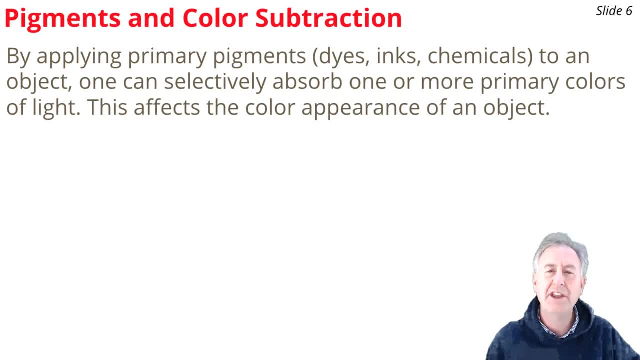 across from them. That's blue light. So there's your three primary pigments. Each one absorbs a single primary color of light. So here's how this idea of color subtraction and pigments work. When you apply a pigment to an object- a sheet of paper, a shirt, whatever it is- that pigment will. 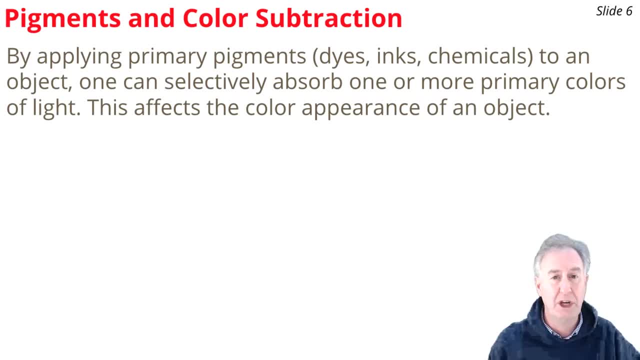 absorb a single primary color of light. So let's just say we have a shirt and magenta pigments in the shirt And we shine white light down on the shirt. White lights, red and green and blue light combined And when it hits that shirt- you remember the color wheel- the magenta will absorb the green. 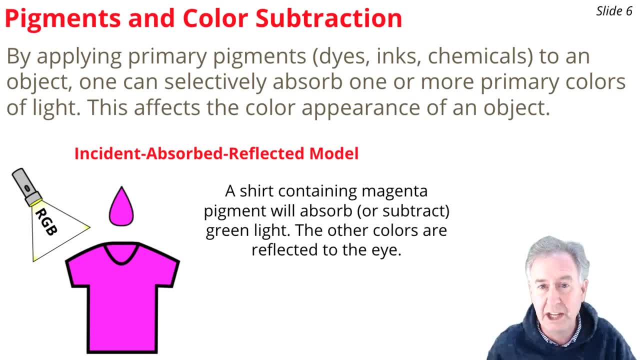 light. So if you start with red, green and blue and green gets taken away, there's two colors remaining: Red and blue. reflect off the shirt to your eye and your eye and your brain work together to say: hey, that's a magenta shirt. 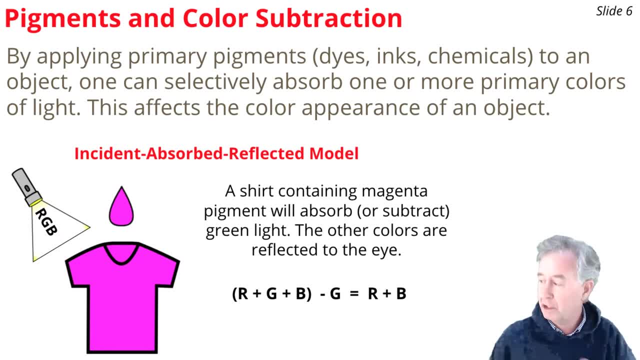 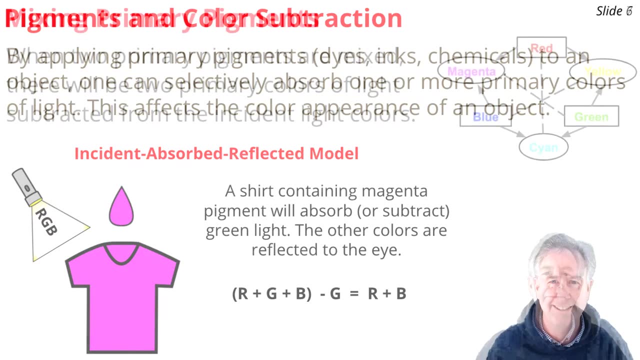 In terms of a color subtraction equation, it would look something like this: You start with red plus green plus blue, But then the shirt takes away the green, so we subtract it, Then do the math. What's left is red plus blue And that kind of light that's equivalent to magenta. So a primary. 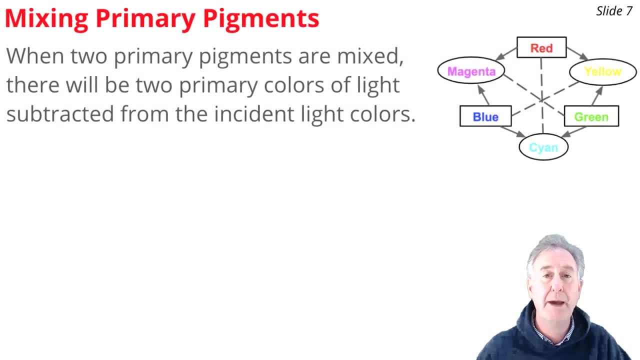 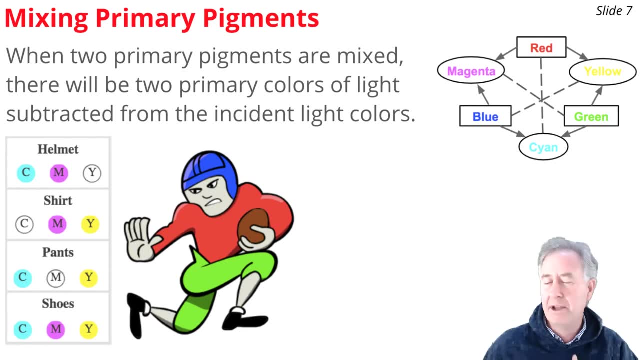 pigment absorbs a single primary color of light. But what happens if you have two or more pigments imparted to, say, an article of clothing? Well, I'm going to tell you what happens. Notice here we have the first color, And then the second color, And then the third color, And then the fourth color. 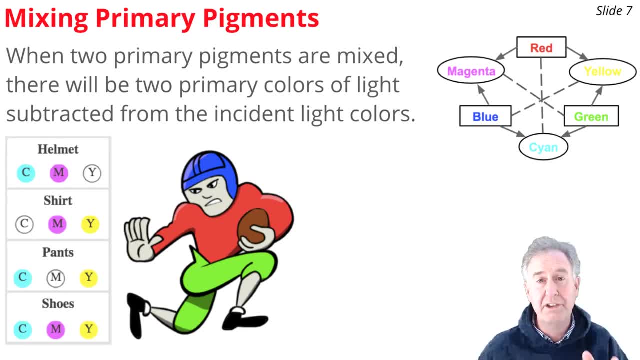 And to the left of the football player is a table that lists the primary pigments imparted to four parts of that uniform. We'll start with the helmet. In the helmet is cyan and magenta pigment. Now if we look above, we'll notice that the cyan pigment is going to absorb red light and the magenta 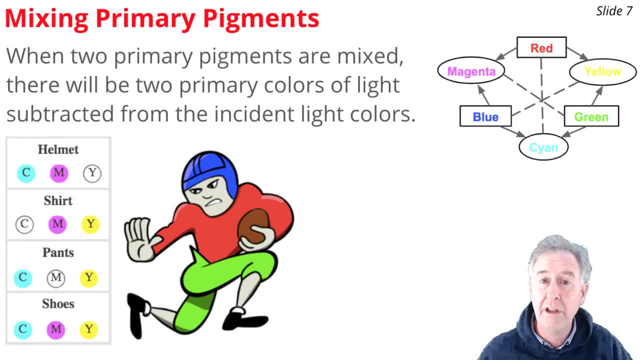 pigment is going to absorb the green light. There's only one color of light that did not get absorbed by that helmet, and it's blue light. It gets reflected. Now let's look at the jersey. The jersey has magenta and yellow pigments, And then the third color, And then the fourth color, And then the. 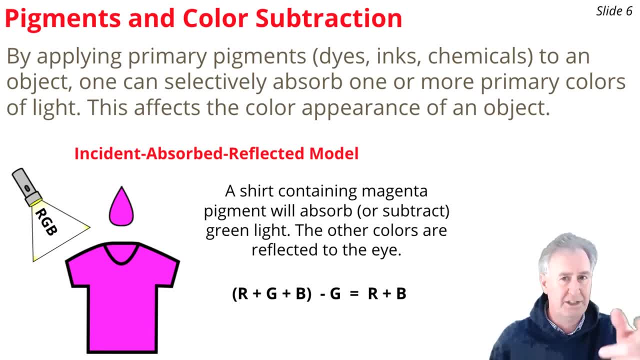 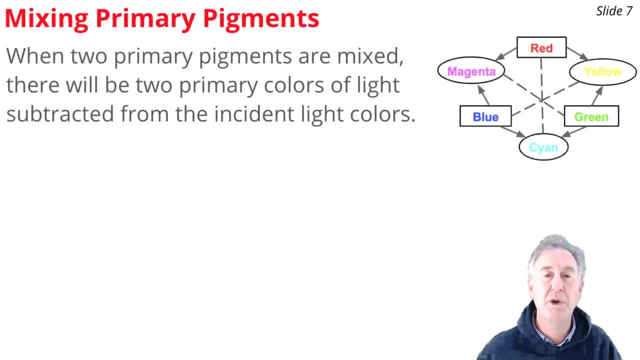 What's left is red plus blue And that kind of light that's equivalent to magenta. So a primary pigment absorbs a single primary color of light. But what happens if you have two or more pigments imparted to, say, an article of clothing? Well, I'm going to tell you what happens. Notice, here we 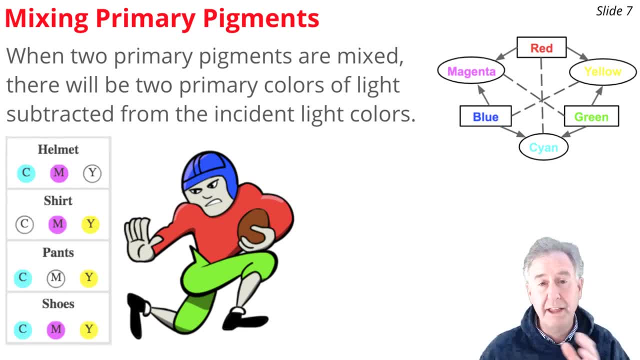 have a football player And to the left of the football player is a table that lists the primary pigments imparted to four parts of that uniform. We'll start with the helmet. In the helmet, the cyan and magenta pigment. Now 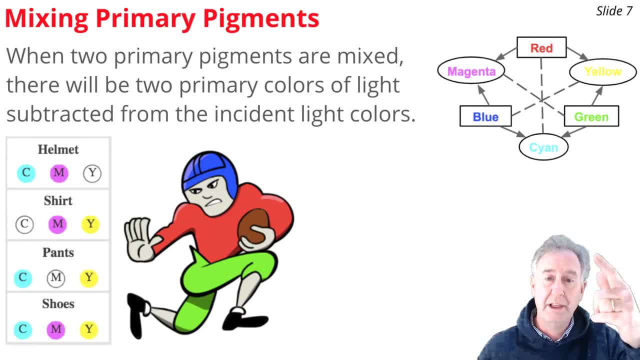 if we look above, we'll notice that the cyan pigment is going to absorb red light and the magenta pigment is going to absorb the green light. There's only one color of light that did not get absorbed by that helmet, and it's blue light. It gets reflected. Now let's look at the jersey, The 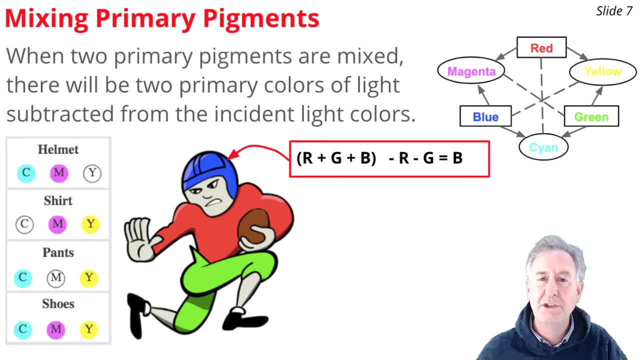 jersey has magenta and yellow pigments imparted to it. So if you look above, you'll notice that the jersey has magenta and yellow pigments imparted to it, And so the magenta is going to absorb the green, The yellow is going to absorb the blue. There's only one primary color of light, not 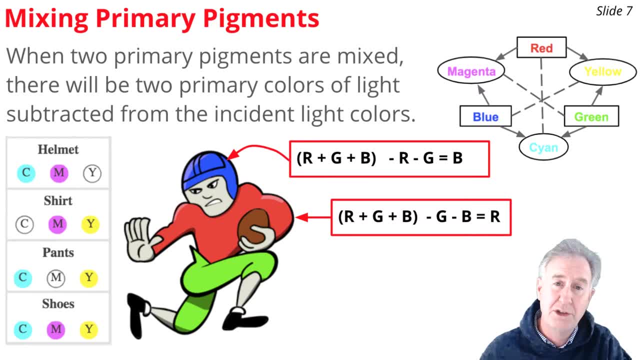 absorbed and it's red light. It gets reflected to your eye and that jersey looks red. Now let's look at the pants. The pants have cyan and yellow pigment on it. The cyan pigment absorbs the red light. The yellow pigment absorbs the blue light. You use the color wheel to figure that out. 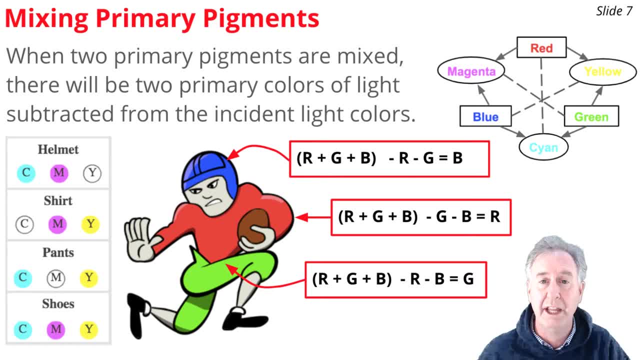 There's only one color of light remaining, and that's green light, And so those pants look green because the other two primary colors of light were absorbed. Now what happens? if you apply all three pigments, Each one absorbs a primary color of light. When you're done, there's no light. 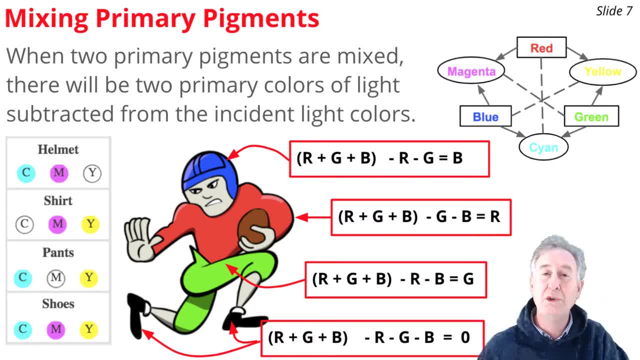 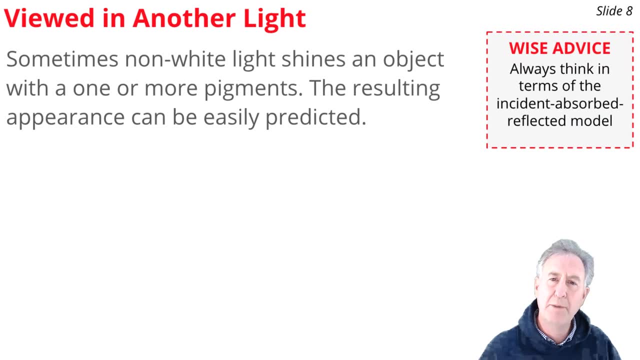 left, Nothing reflects to your eye and those shoes look black. Black is the absence of colors of light, And so this explains the various rules of color subtraction when you have two or more pigments imparted to an object. The first rule with the football uniform had to do with white light shining on the various parts of 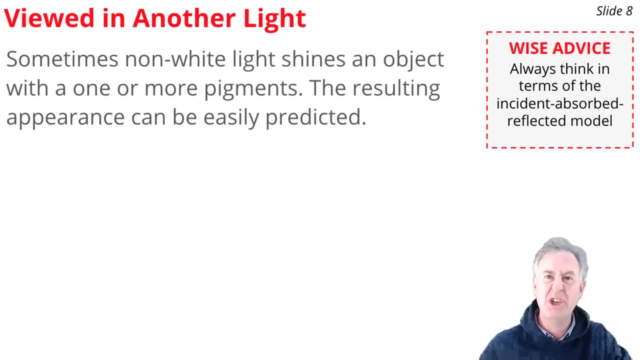 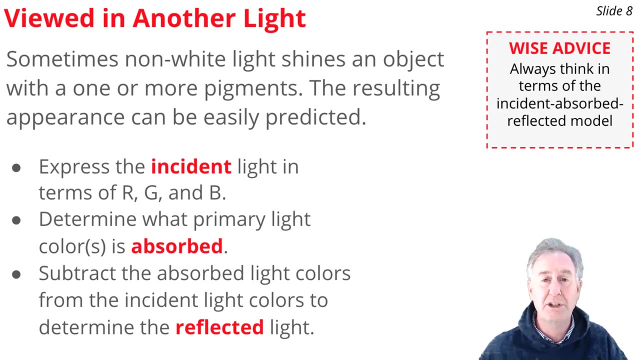 the uniform. Well, what happens if it's not white light? What if it's yellow light, magenta light, cyan light? Well, you do the same thing. You have to use the incident-absorbed-reflected model, and it begins by asking what primary colors of light are. incident on that object, Express it in. 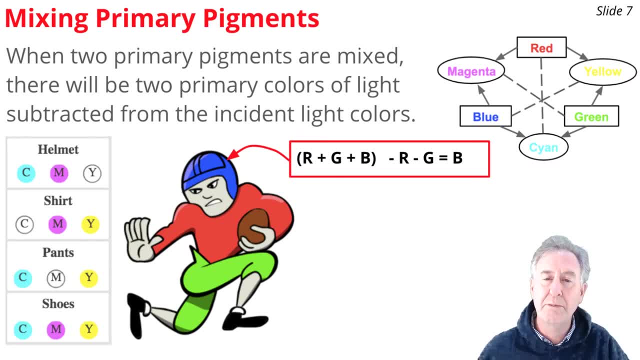 ring is beings pink pigments imparted to it, And so the magenta is going to absorb the green, The yellow is going to absorb the blue. There is only one primary color of light not absorbed, And it's red light. It gets reflected to your eye and that jersey looks red. Now let's look at the pants. 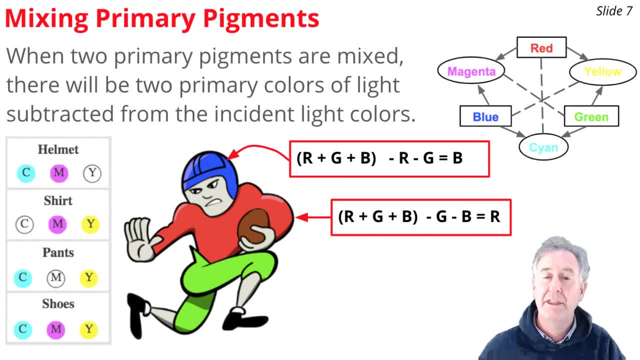 The pants have cyan and yellow pigment on it. The cyan pigment absorbs the red light. The yellow pigment absorbs the blue light. Here's a color wheel. figure that out. There's only one color of light remaining and that's green light. So on the mid-utation we have blue light. 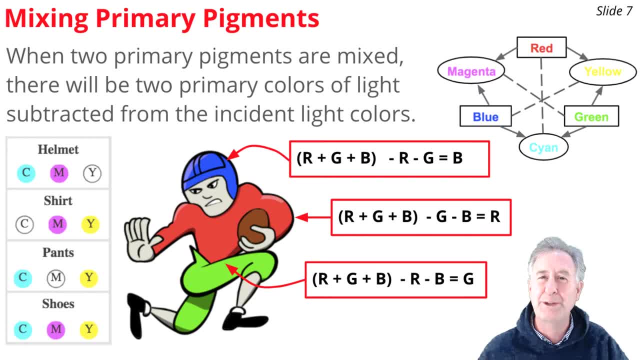 pants look green because the other two primary colors of light were absorbed. Now what happens if you apply all three pigments? Each one absorbs a primary color of light. When you're done, there's no light left, Nothing reflects to your eye and those shoes look black. Black is the absence of 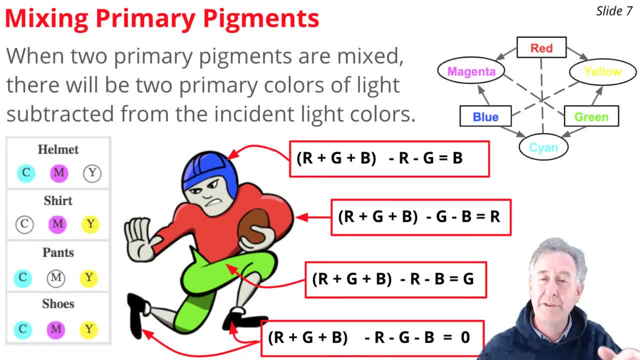 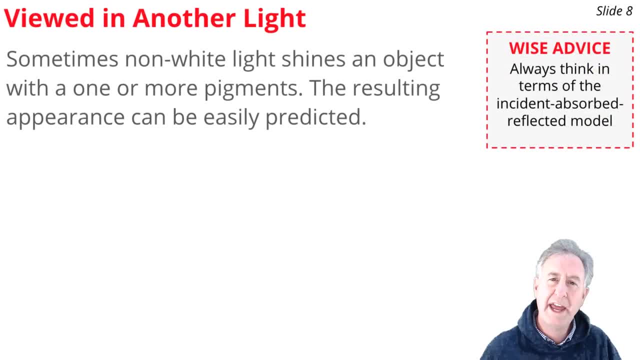 colors of light, and so this explains the various rules of color subtraction when you have two or more pigments imparted to an object. So that example with the football uniform had to do with white light shining on the various parts of the uniform. Well, what happens if it's not white light? 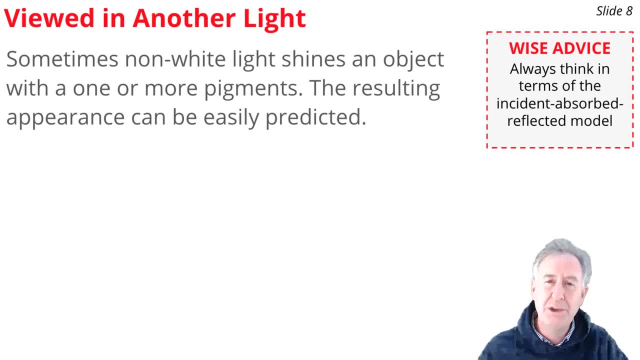 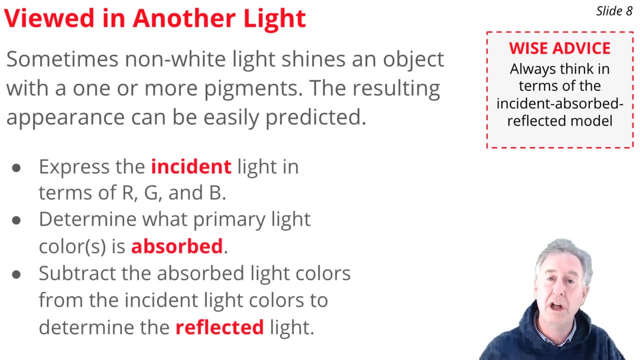 What if it's yellow light, magenta light, cyan light? Well, you do the same thing. You have to use the incident absorbed, reflected model, and it begins by asking what primary colors of light are incident on that object, Express it in terms of red, green and blue. Then you look at the pigment. 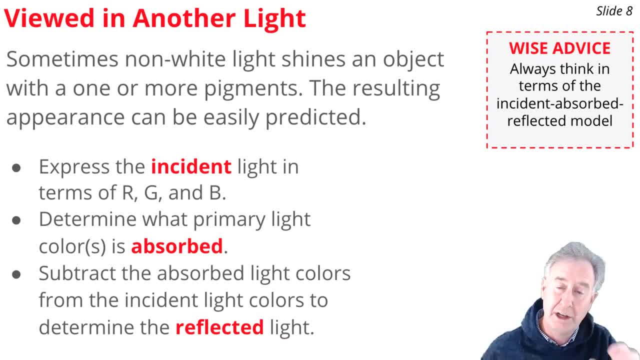 and you use a color wheel to figure out which of the incident colors of light get absorbed. Finally, subtract the absorbed light colors from the incident light colors to see what's remaining. That's the light that gets reflected to your eye and determines the color appearance of that object. 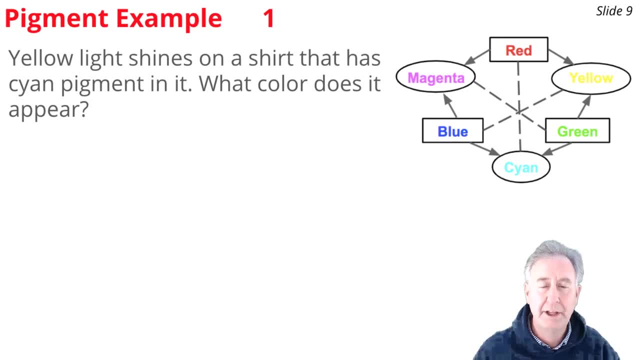 So let's use this incident absorbed reflected model and this color schematic to answer this question. It says: yellow light shines on a shirt that has cyan pigment in it. What color does the shirt appear? So here's our situation: Yellow light shining on a shirt with cyan pigment. The yellow light is simply red plus green light, So the red 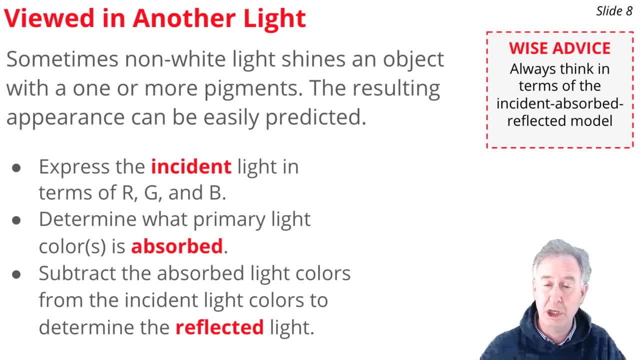 terms of red, green and blue. Then you look at the pigment and you use a color wheel to figure out which of the incident colors of light get absorbed. Finally, subtract the absorbed light colors from the incident light colors to see what's remaining. 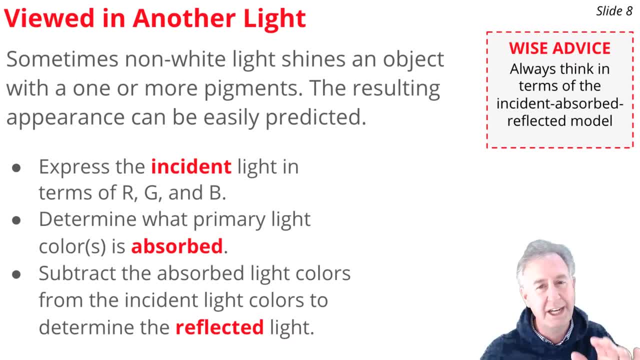 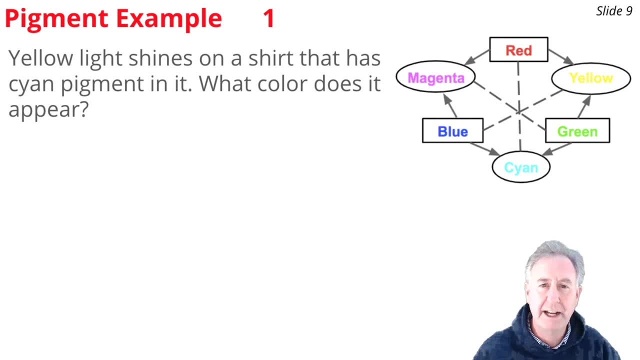 That's the light that gets reflected to your eye and determines the color appearance of that object. So let's use this incident-absorbed-reflected model and this color schematic to answer this question. It says: yellow light shines on a shirt that has cyan pigment in it. What color does the shirt appear? 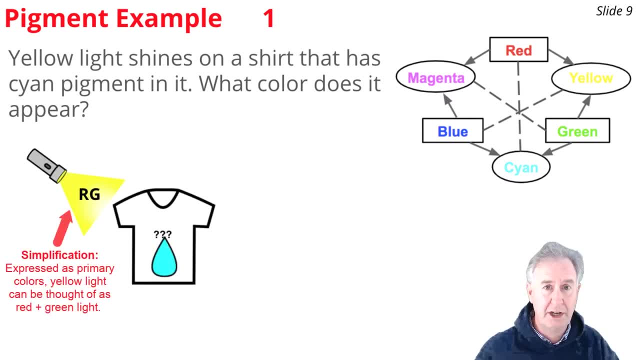 So here's our schematic situation: Yellow light shining on a shirt with cyan pigment. The yellow light is simply red plus green light. So the red plus green light hits the shirt and it's got cyan pigment And cyan can absorb red. So the red gets taken away and the green light gets reflected to my eye. I look at: 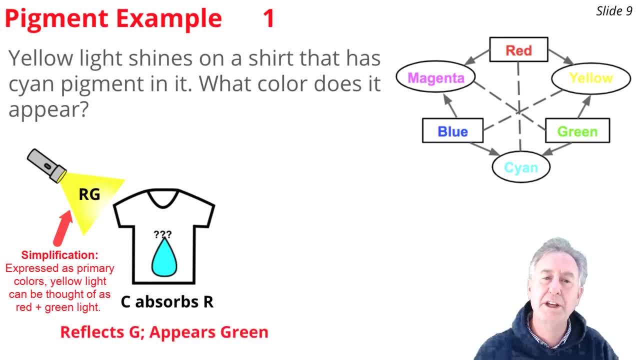 that shirt and it looks green to me. So if we were to express this with a color equation, we put it something like this: We start with the incident light color R plus G, That's yellow. We subtract the absorbed light color Cyan absorbs red. So I go minus R And then I do the math: Red plus green. 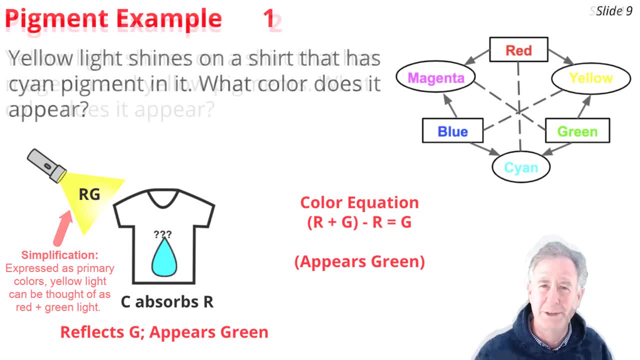 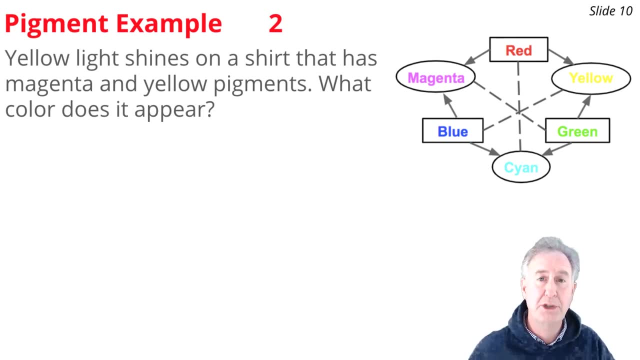 minus red equal green. That shirt appears green. Here's example number two: Yellow light shines on a shirt that has two pigments in it: magenta and yellow pigment. What color does that shirt appear? So here's the situation: We have yellow. 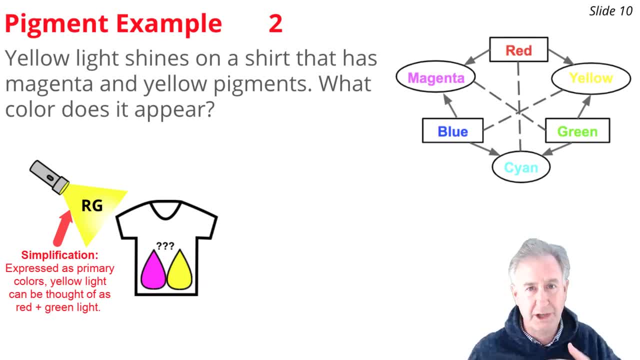 light, which is simply red plus green light. incident on the shirt. Those are my incident colors. The shirt contains yellow and magenta pigment. Now if we look above, the magenta will take away the green and green shining on that shirt. so I have to subtract the green because 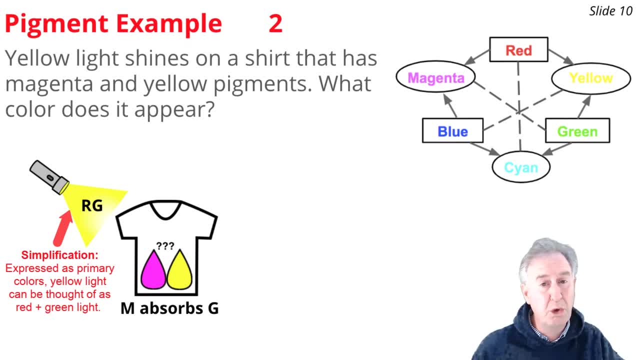 it gets absorbed. Now the yellow would absorb blue, but there's no blue light here, so we don't have to worry about the yellow pigment. The red light's going to get reflected to my eye. when I look at this shirt. it looks red. Here's the color equation. I start with yellow light. that's r plus. 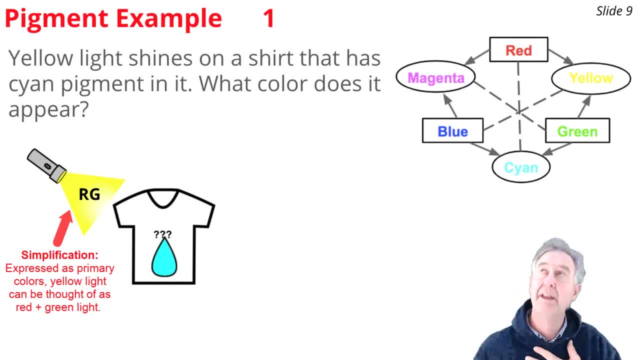 plus green light hits the shirt and it's got cyan pigment and cyan can absorb red. So the red gets taken away and the green light gets reflected to my eye. I look at that shirt and it looks green to me. So if we were to express a color wheel that has cyan pigment in it, what color does the shirt appear? 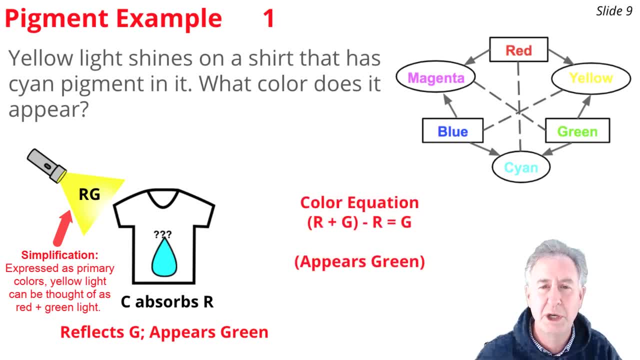 So we're going to express this with a color equation. We put it something like this: We start with the incident light color r plus g, That's yellow. We subtract the absorbed light color, Cyan absorbs red. so I go minus r And then I do the math: Red plus green, minus red, equal green. That shirt appears green. 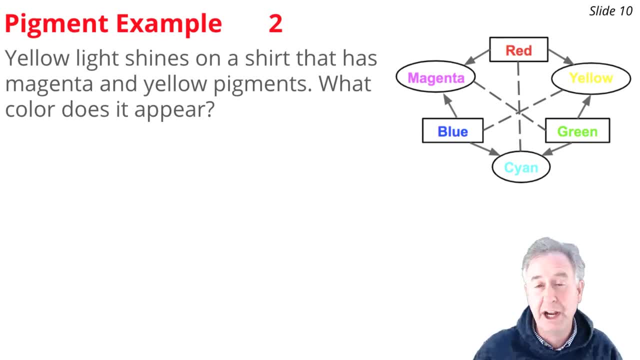 Here's example number two: Yellow light shines on a shirt that has two pigments in it: Magenta and yellow pigment. What color does that shirt appear? So here's the situation: We have yellow light, which is simply red, plus green light. incident on the shirt. 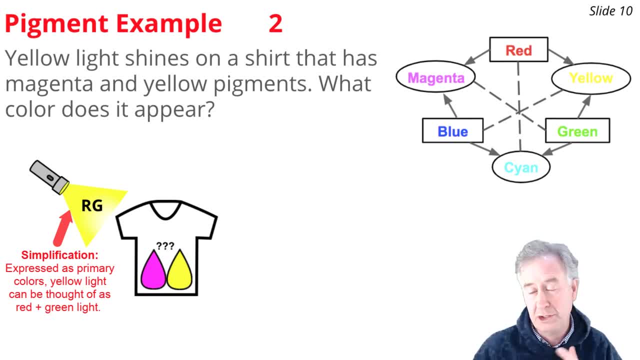 Those are my incident colors. The shirt contains yellow and magenta pigment. Now, if we look above, the magenta will take away the green and green is shining on that shirt, So I have to subtract the green because it gets absorbed. Now the yellow would absorb blue, but there's no blue light here, So we don't have to worry about the yellow pigment. 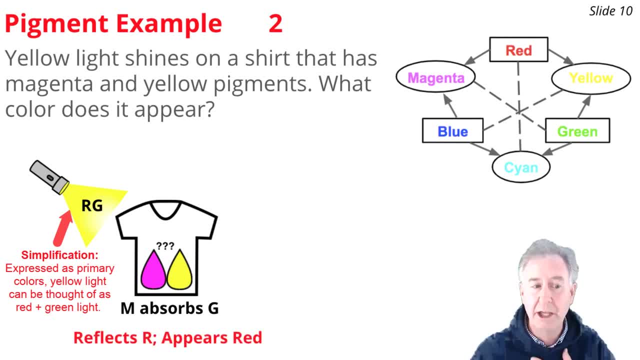 The red light's going to get reflected to my eye When I look at this shirt. it looks red. Here's the color equation. I start with yellow light. that's R plus G. I take away the green light minus G. 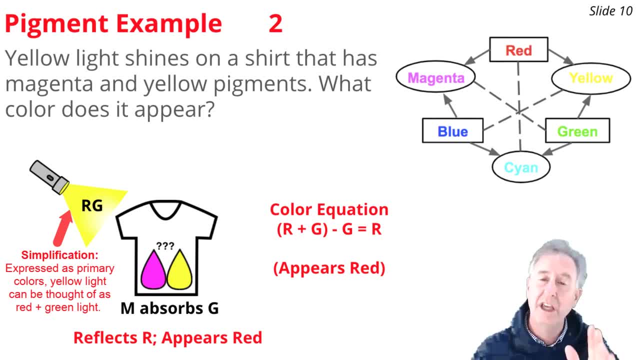 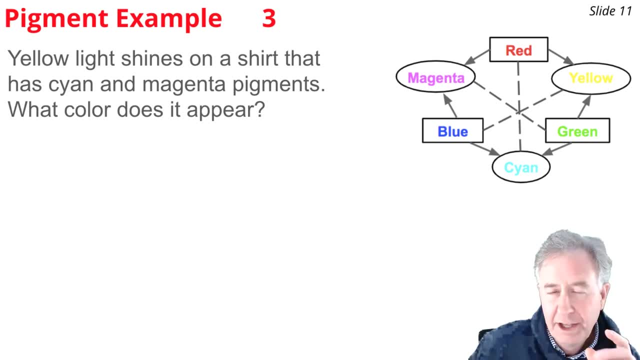 I do the math: R plus G minus G equal R. This shirt appears red. So here's our final example: Yellow light shines on a shirt that has cyan and magenta pigments in it. What color does the shirt appear? So my situation is this. 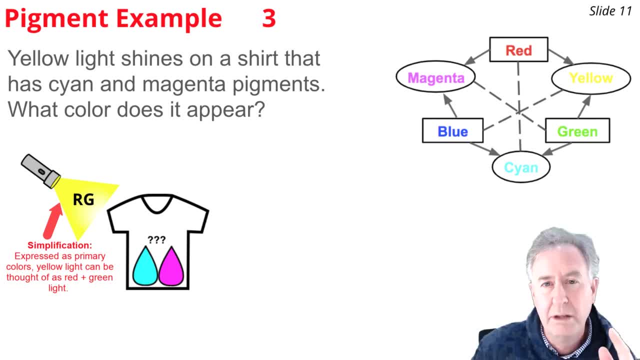 I have yellow light- I'm starting with incident light colors of red plus green- And it's shining on a shirt with two pigments: The cyan pigment absorbs red light And the magenta pigment it absorbs green light. That's the only light that's shining on this shirt. 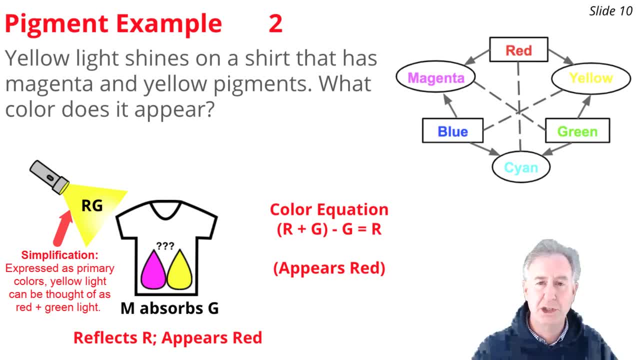 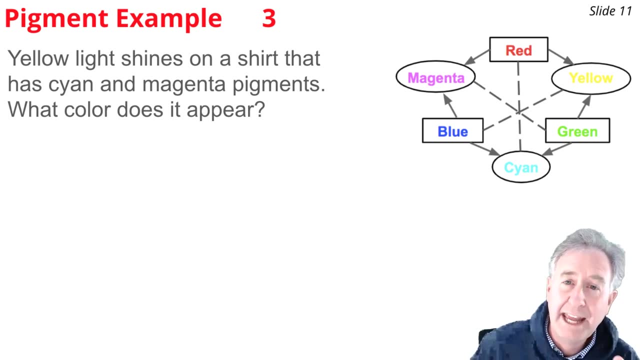 g. I take away the green light, minus g. I do the math: r plus g minus g equal r. This shirt appears red. So here's our final example: Yellow light shines on a shirt That has cyan and magenta pigments in it. What color does the shirt appear? So my situation is: 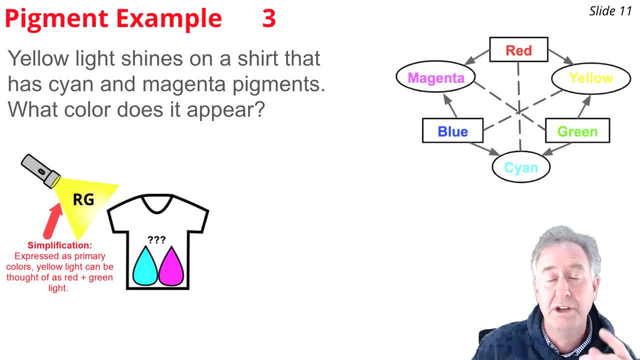 this. I have yellow light- I'm starting with incident light colors of red plus green- and it's shining on a shirt with two pigments: The cyan pigment absorbs red light and the magenta pigment it absorbs green light. That's the only light that's shining on the shirt, So 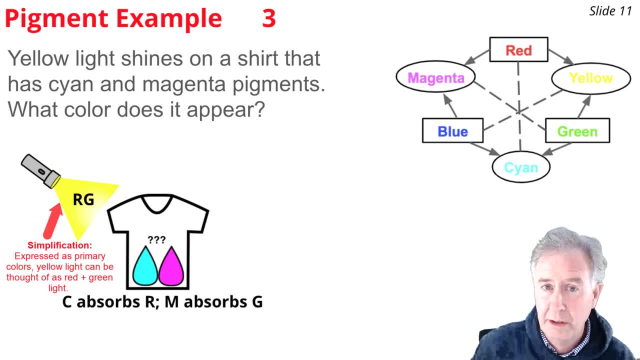 I start with red plus green and the red gets absorbed and the green gets absorbed, The shirt's black, There's nothing left, No light can reflect because it all gets absorbed and this shirt looks black. Here's the color equation: I start with red plus green and then I subtract red, because 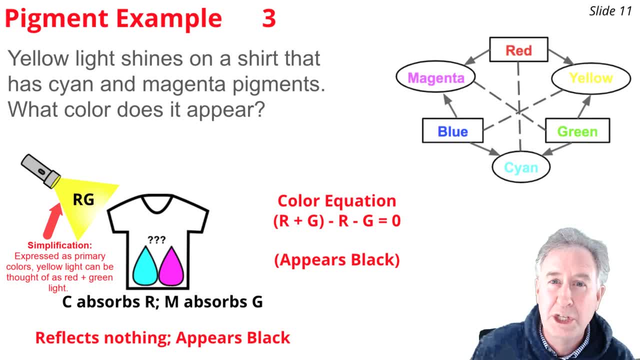 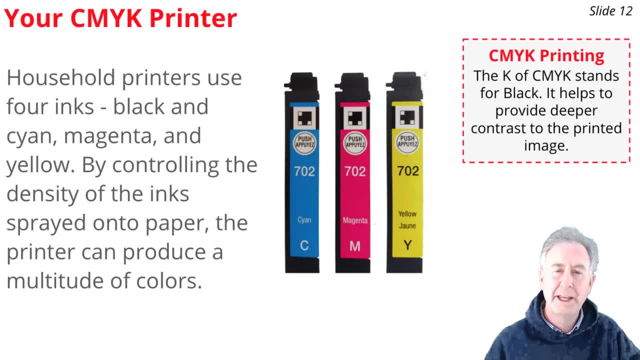 the cyan pigment's there, and then I subtract green, the work of magenta pigment and what's left is zero and this shirt looks black. So in the world of printers and printing and paper-based publishing, the most common model is the CMYK printing process. 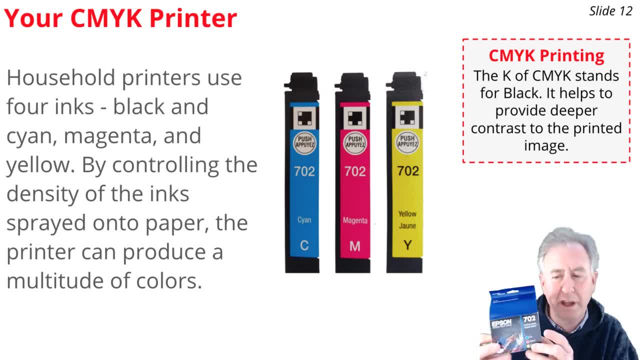 I just replaced the ink in my color printer the other day and this is the box, and that's what the side of the box looks like. You see it right here. I replaced the ink in my color printer with cyan ink, magenta ink and yellow ink. These are the primary pigments. Each one of these pigments. 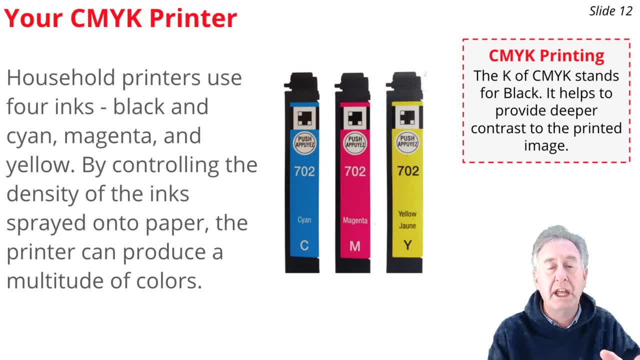 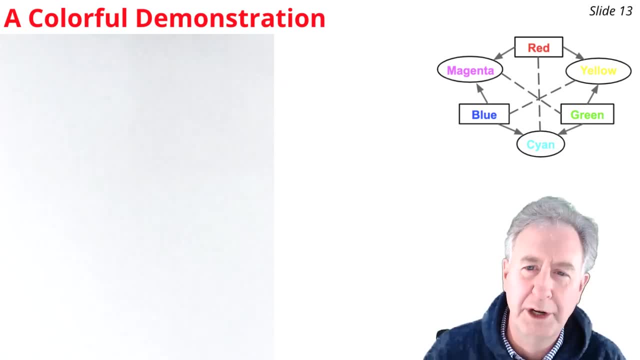 Now watch this. I want to use my CMYK printer to create that image, and so I'm going to use three inks: I'm going to use the cyan ink, the magenta ink and I'm going to use the yellow ink. 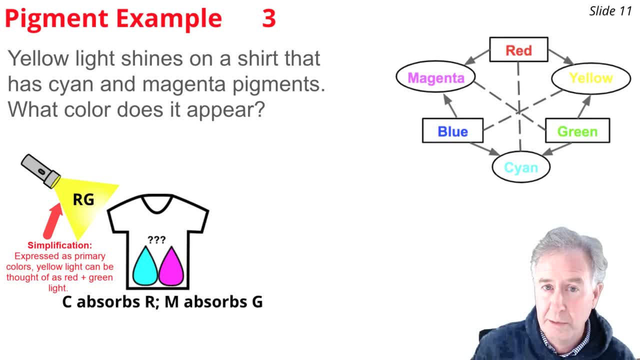 So I start with red plus green, And the red gets absorbed And the green gets absorbed. There's nothing left, No light can reflect because it all gets absorbed And this shirt looks black. Here's the color equation: I start with red plus green. 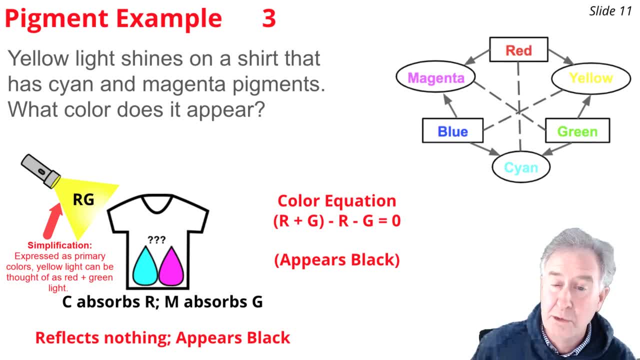 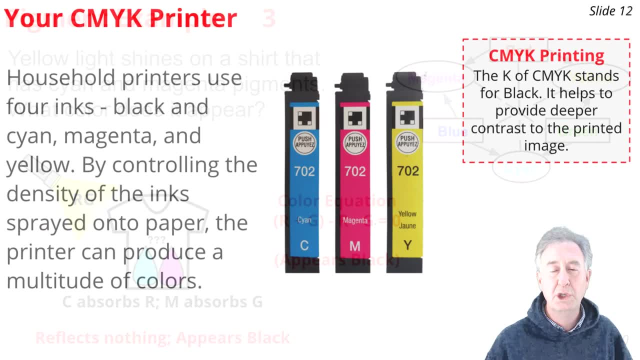 And then I subtract red because the cyan pigment's there, And then I subtract green, the work of magenta pigment, And what's left is zero And this shirt looks black. So, in the world of printers and printing and paper-based publishing, 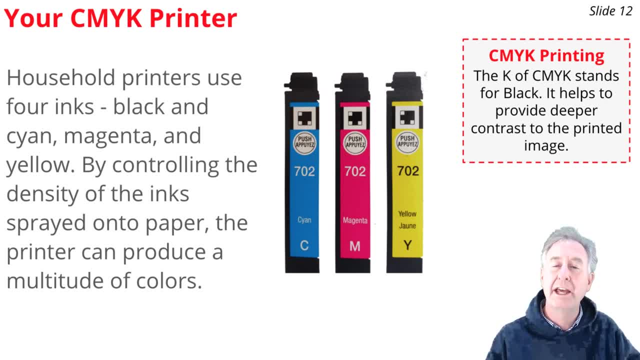 the most common model, which is the CMYK printing process. I just replaced the ink in my color printer the other day And this is the box, And that's what the side of the box looks like. You see it right here. 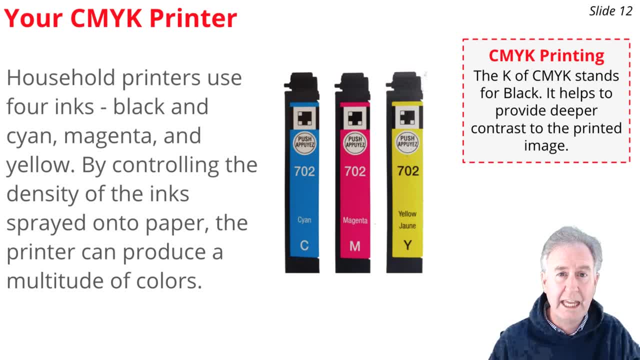 I replaced the ink in my color printer with cyan ink, magenta ink and yellow ink. These are the primary pigments. Each one of these pigments absorbs a primary color of light And by using all three you can take away as you need to create any printed image you want. 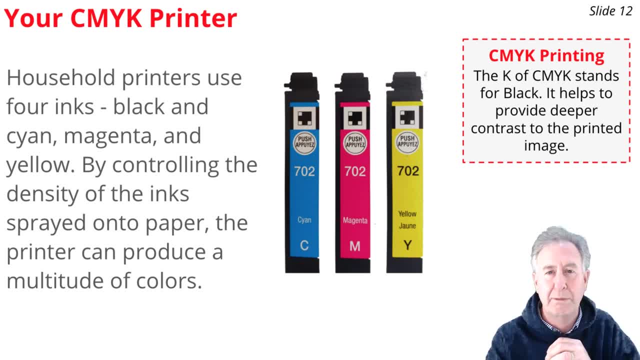 And by using all three, you can take away as you need to create any printed image you want. You can take away as you need to create any printed image you want. The K in this process stands for black, And the black is simply used to give a little deeper contrast to the printed image. 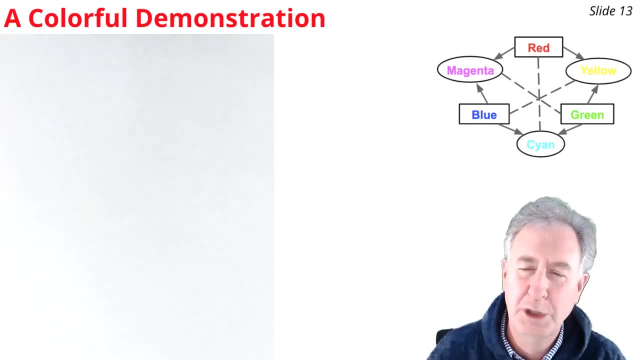 Now watch this. I want to use my CMYK printer to create that image, And so I'm going to use three inks. I'm going to use the cyan ink, a magenta ink, and I'm going to use the yellow ink. 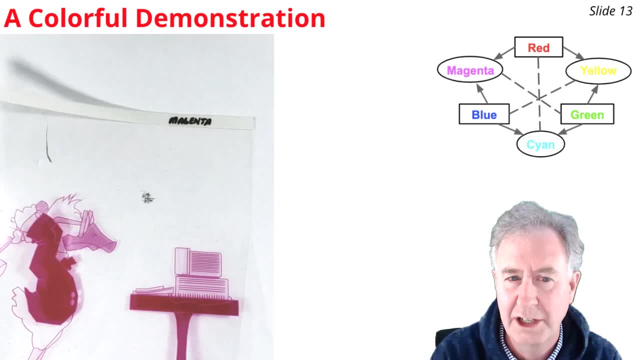 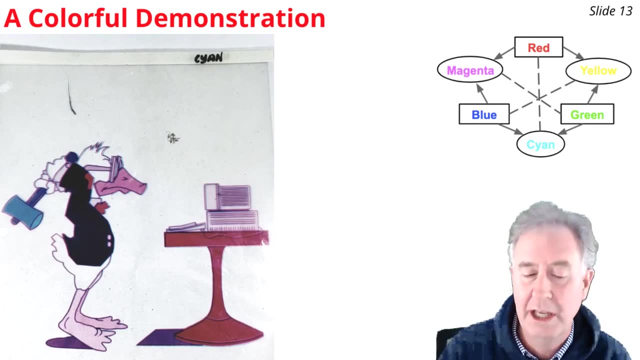 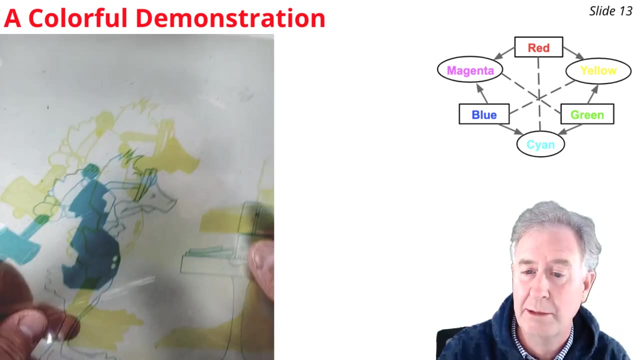 And I'm going to mix them with various ink intensities to produce that original image. So here's the result of mixing cyan and magenta inks and you'll notice you get a lot of blues. Now I'm going to take the cyan and the yellow ink and mix those and wherever they overlap I end up getting some greens. 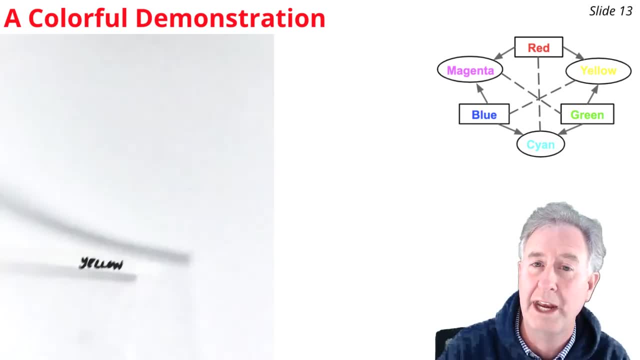 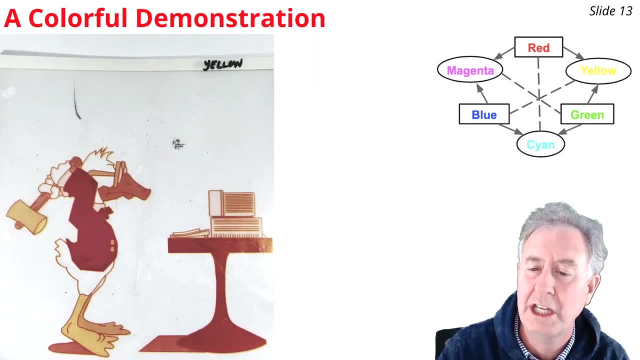 The green results because the cyan takes away the red and the yellow takes away the blue light. Now I'm going to take the yellow ink and mix it with the magenta ink, and that's where I get a lot of the reds.